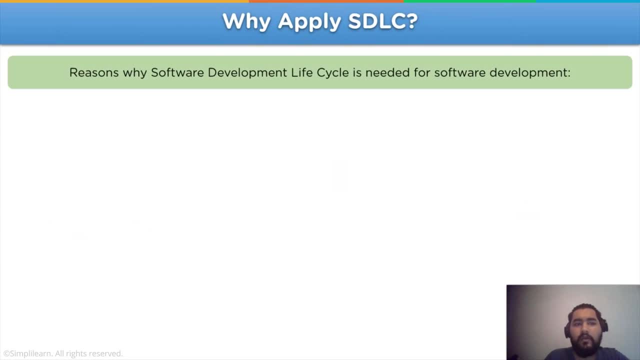 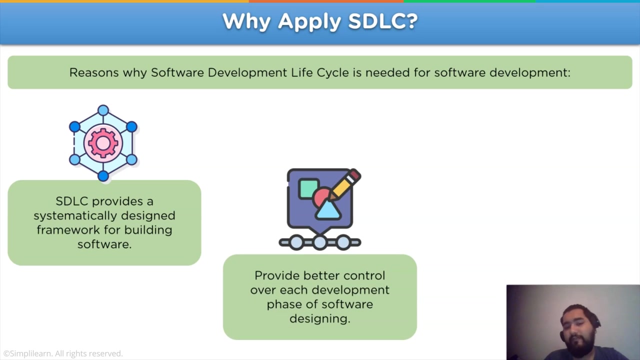 apply the SDLC cycle. The reason to apply the SDLC lifecycle in the development of a software is because it provides a team with a developed lifecycle format or a framework to build a software from scratch. It provides better control over each development phase of the software designing. 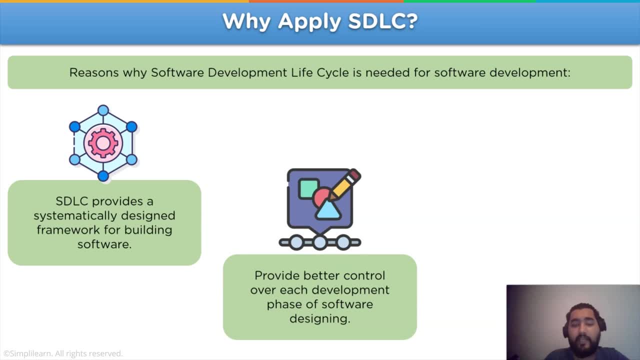 Where the coding is to be done. what about the errors in the development and different particular points or attributes? These are important to understand while designing a attributes that affect the functioning of a software. It also improves client interaction with the multiple development phases of the software. 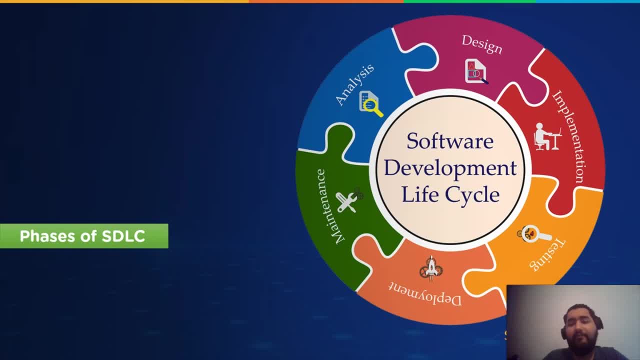 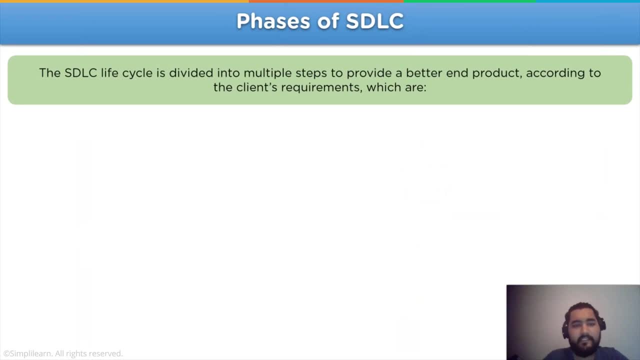 Now let's move on to the next heading, that is, different phases that involve the development of a software. The SDLC lifecycle is divided into multiple steps to provide a better end product according to the client's request, which are planning and requirement analysis. At this step, the planning and the requirement of the software is discussed with the client. 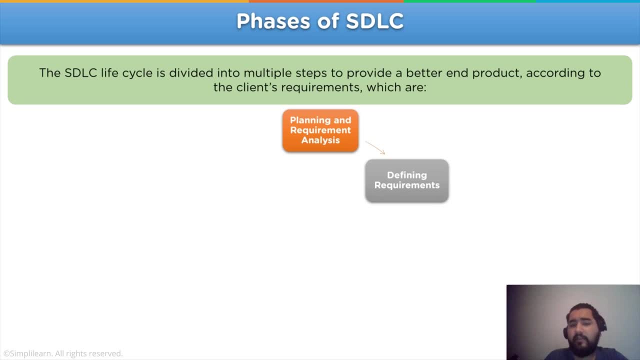 Moving on with defining the requirements. According to the planned scenario, we will define certain terms for development of the software. Continuing with designing the software, coding or implementing the physical points of the software. Moving on to the testing phase, where different scenarios are used to test the overall functioning of a software. As for the last step, we have: 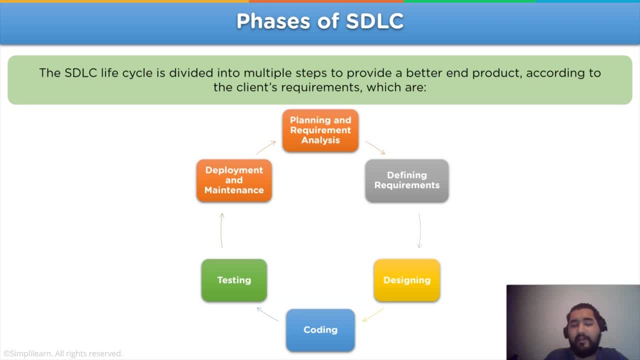 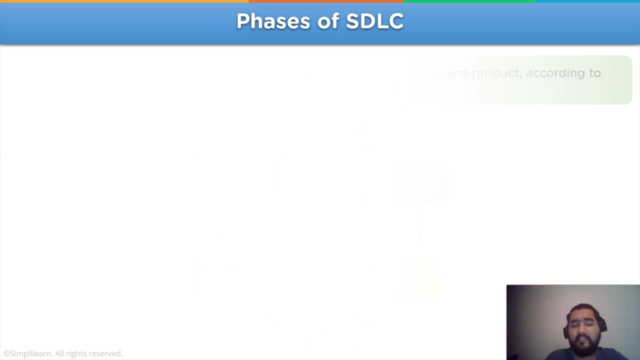 deployment and maintenance, where the developed software is deployed and is assessed by the users to check for any errors or bugs. Moving on, let's take a look at the individual phases of SDLC. The first phase is planning and requirement analysis. Planning is the most important step for software development. The developer performs the requirement analysis. 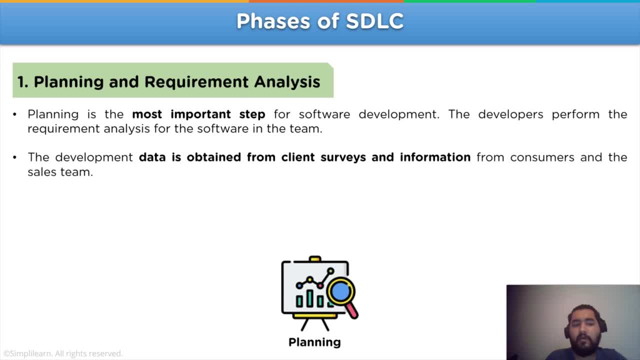 for the software in the team Moving on the software development. data is obtained from client surveys and information which are used from consumers or sales team. The analysis data acts as a basis for planning the development route for the required software. Also, the analysis data is used to check for any risk as for quality assurance of the software being developed at different stages. 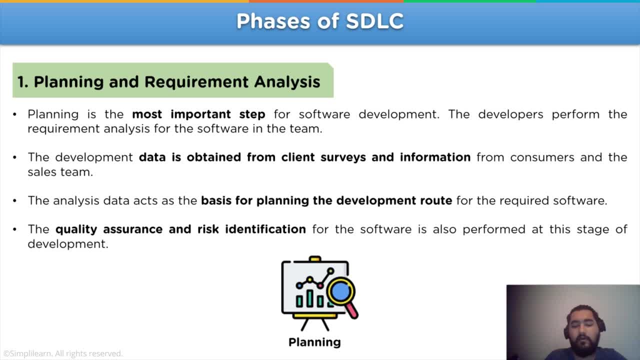 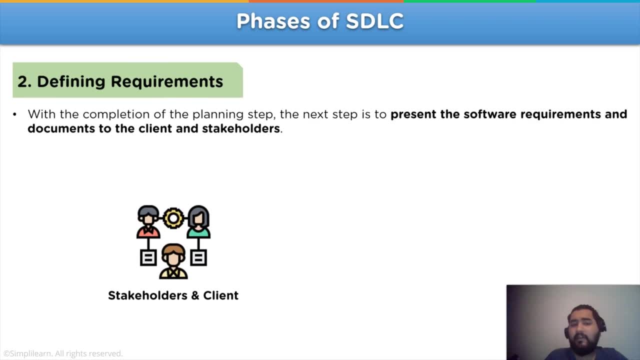 Moving on, we have the second stage, that is, defining requirements. With the completion of planning step, the next step is to present the software requirements and documents to the client and the stakeholders for verification if they are satisfied with the planned scenario. The task of defining requirement is performed by the software requirement specification document, also known as. 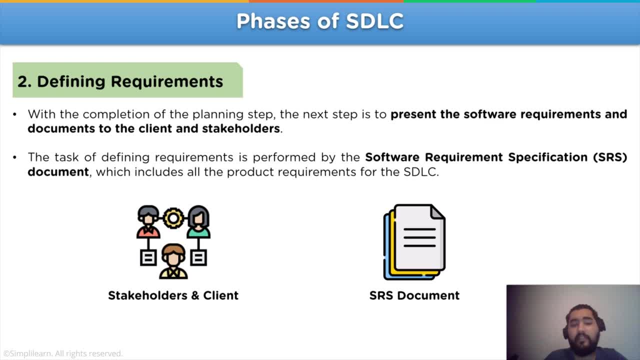 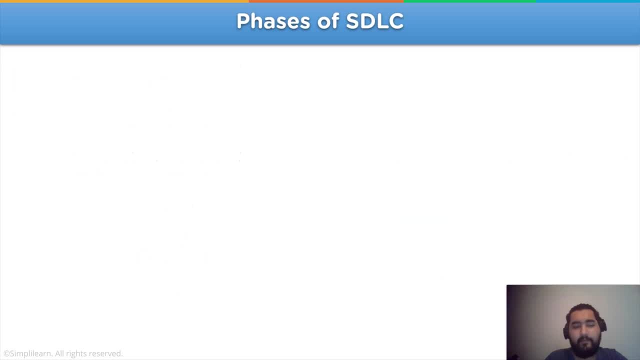 SRS document, which include all the data and information related to the product being developed. Moving on, we have the third step, that is, designing the software. In this step, the SRS document is used by the developer to use the most optimized architecture for the development of the software. 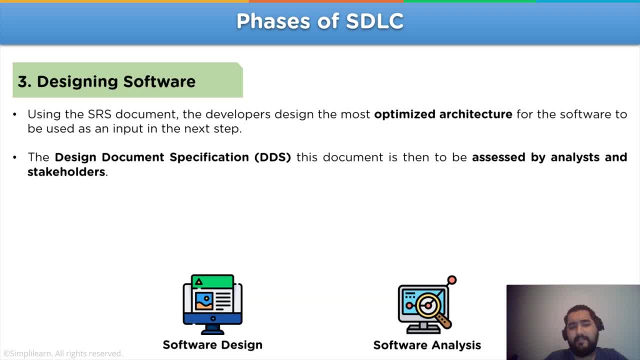 The developed architecture is used using the DDS document, also known as design document. The design document is used by the developer to develop the software. The design document specification, which is shared with the analyst and the stakeholders to check multiple attributes of the software. 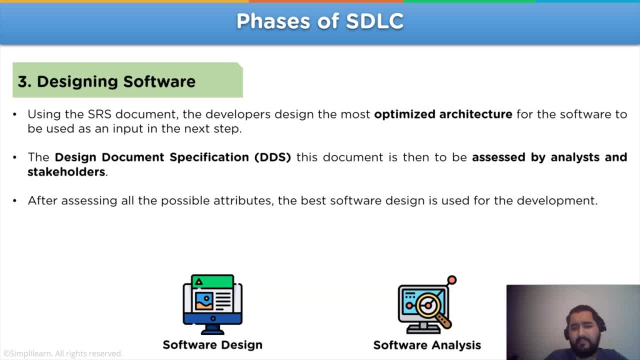 Moving on. after assessing all the possible attributes, the best software design is used for the development. Depending upon the requirements, different designs are used to develop the software. The first one is known as high-level design and the other one is known as low-level design. 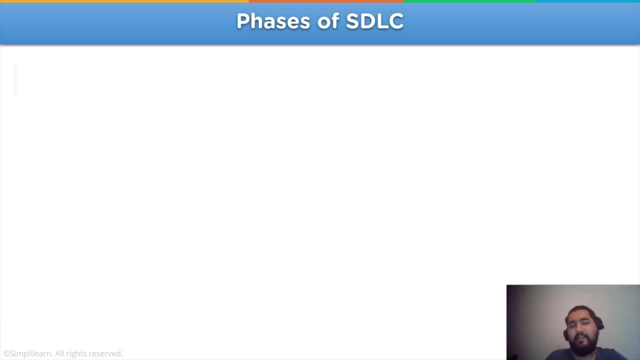 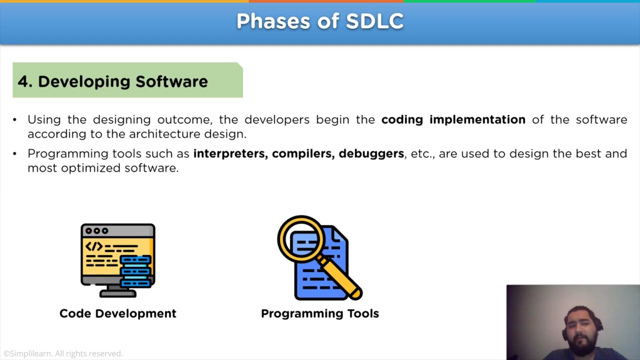 Moving on, let's take a look at the fourth step of SDLC, that is, developing software. Using the designing outcome from the previous step, the developers begin the coding implementation, which is in accordance with the architecture design by the developers. Programming tools such as interpreters, compilers and debuggers are used to design the best and the most organized. 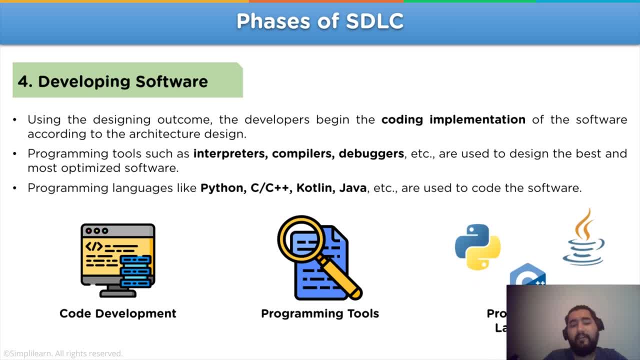 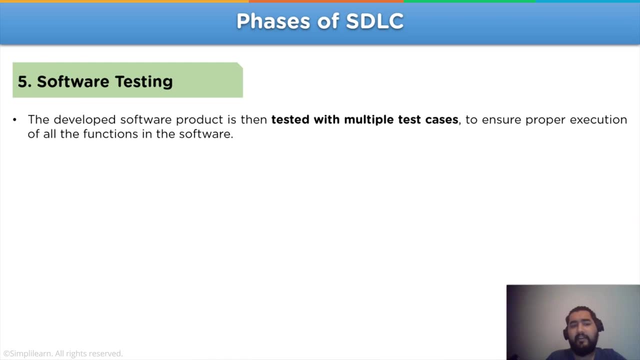 software design. It is developed using multiple languages, for example Python, Kotlin, Java, C. Now let's move on to the next stage, that is software testing. In this stage, the developed software is tested with multiple test cases and different scenarios to ensure proper execution of all the functions included in the software. 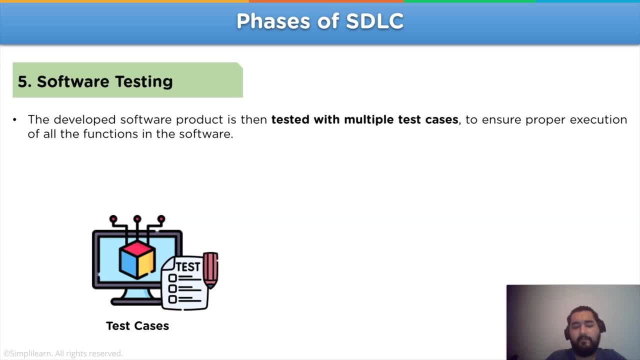 With respect to the testing of a software in SDLC, each phase has multiple case scenarios to assess it. Through all the test cases done, the bugs, errors or the flaws of the software product are fixed that are to meet the requirement of the client, as well as the SRS document.